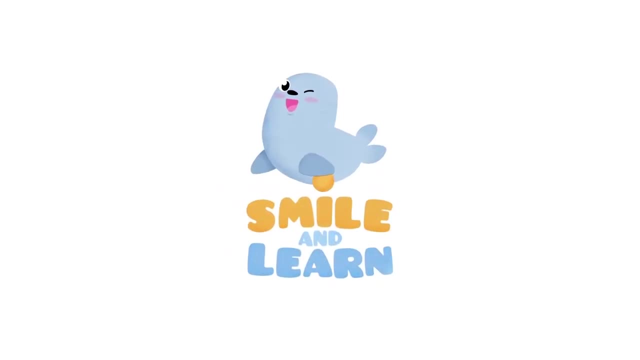 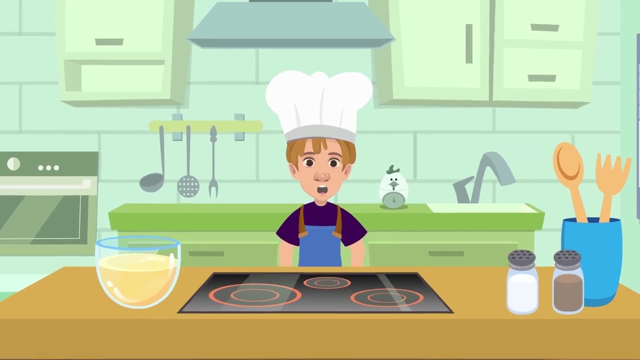 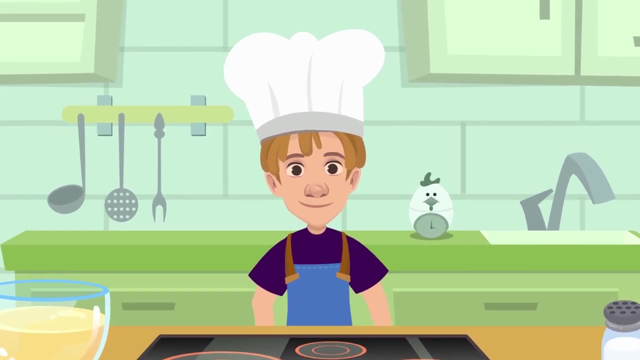 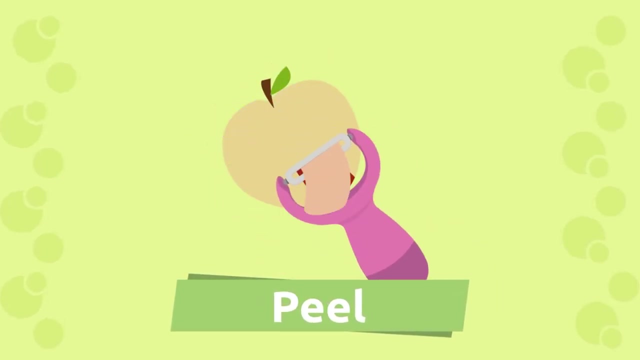 Smile and Learn. Hello friends, Welcome to our cooking class. Today we're going to learn all the cooking verbs you need to know to become a great chef. Ready, Here we go. Peel, Peel, Repeat after me, Peel, Super duper, Chop. 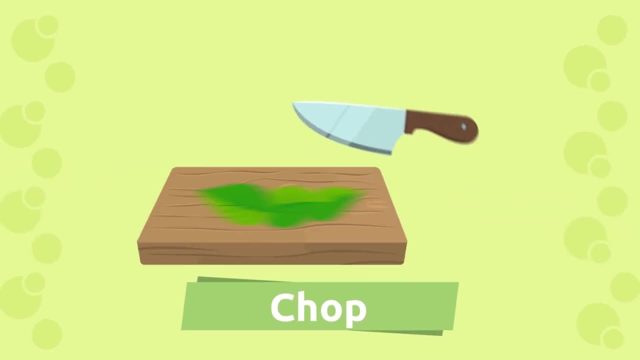 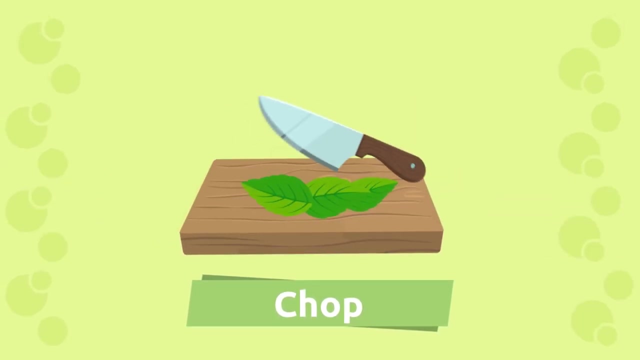 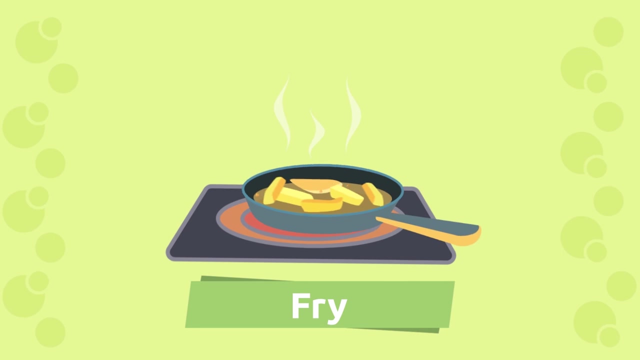 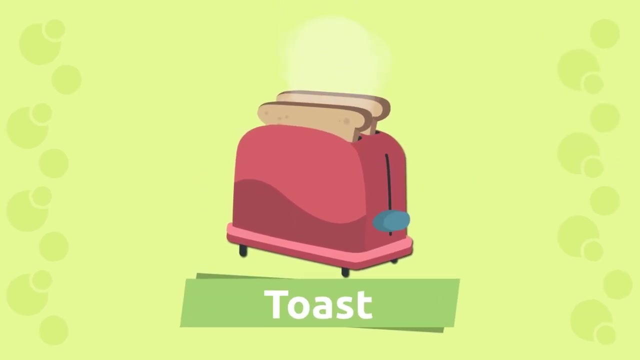 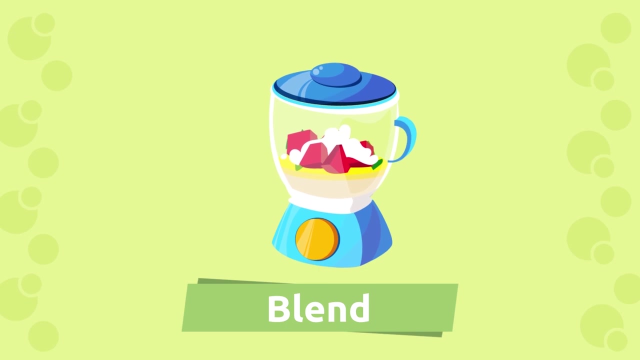 Chop- Repeat after me Chop. Brilliant Fry, Fry. Repeat after me: Fry. Great job. Toast. Toast- Repeat after me: Toast. You're doing so well. Blend, Blend. Repeat after me. Toast, Toast- Repeat after me. Repeat after me: Toast, Toast, Toast, Toast, Toast. 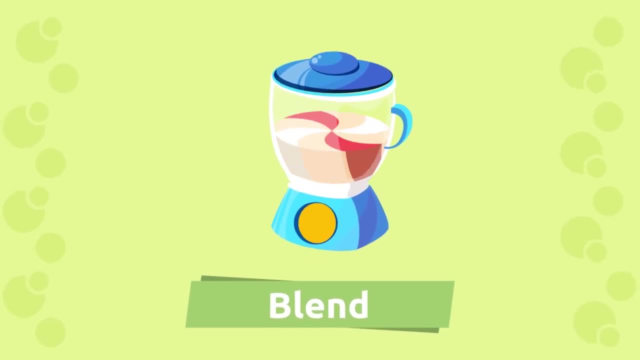 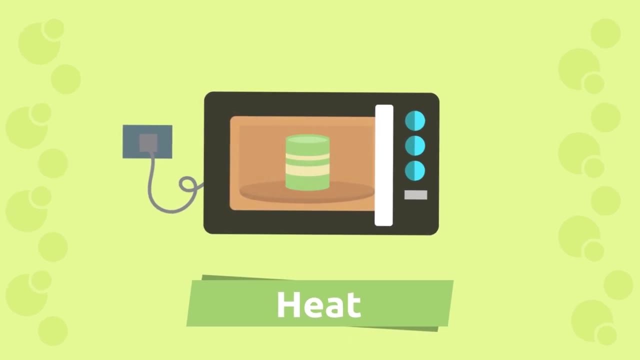 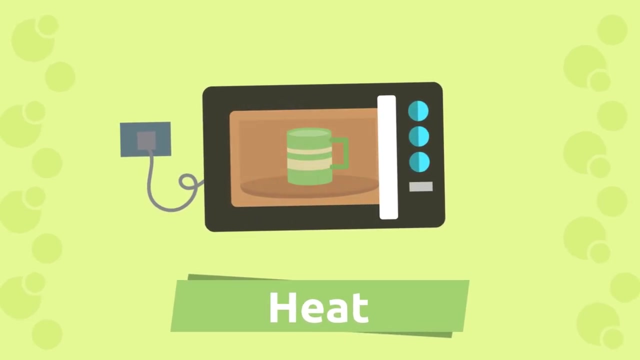 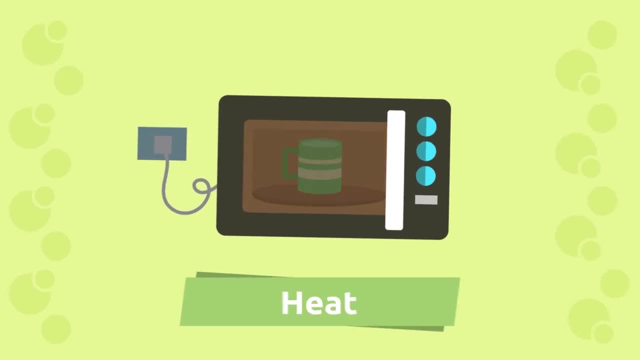 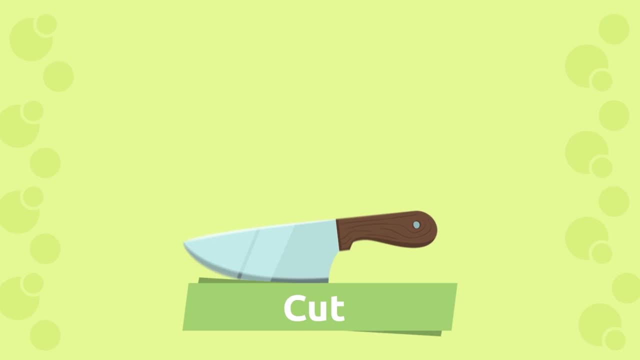 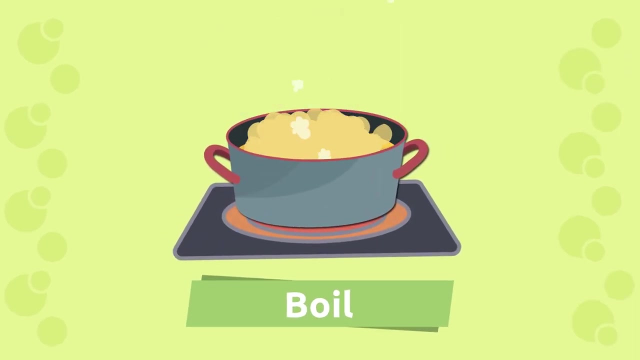 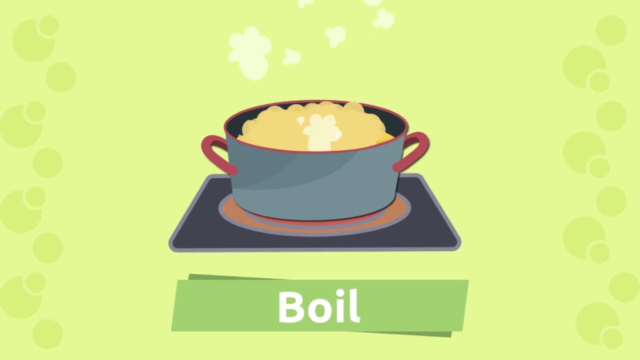 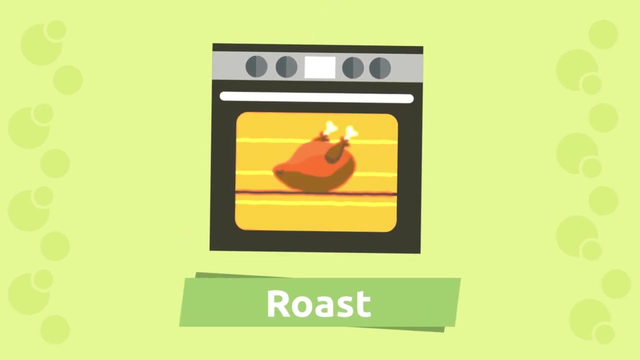 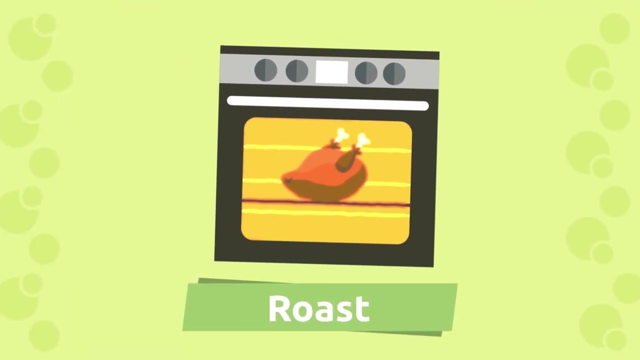 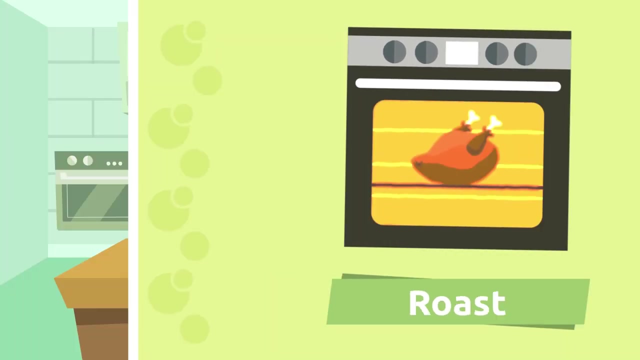 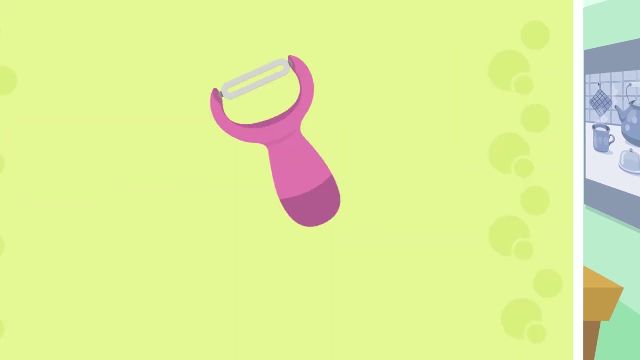 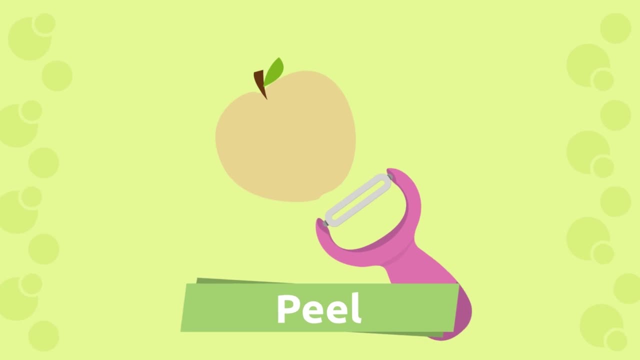 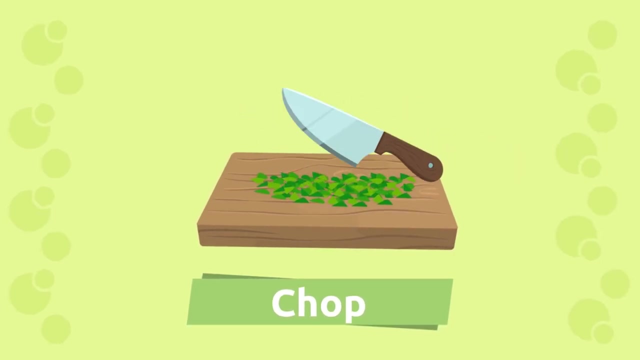 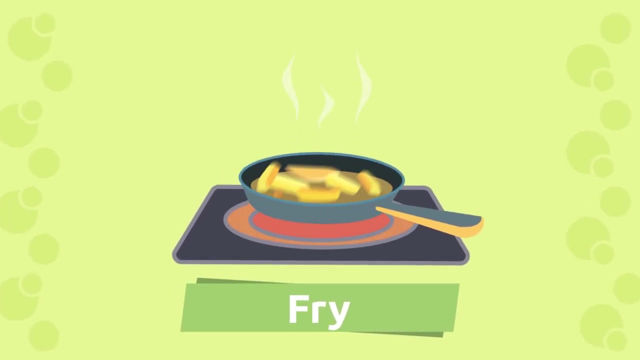 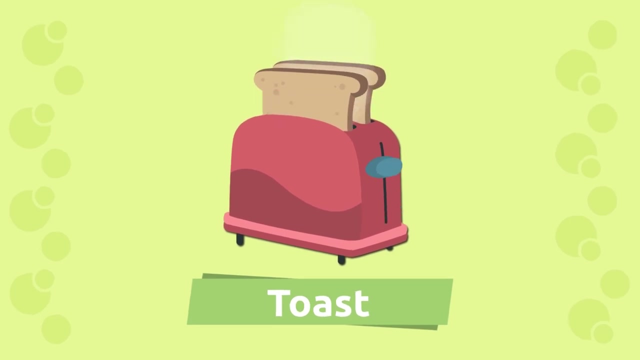 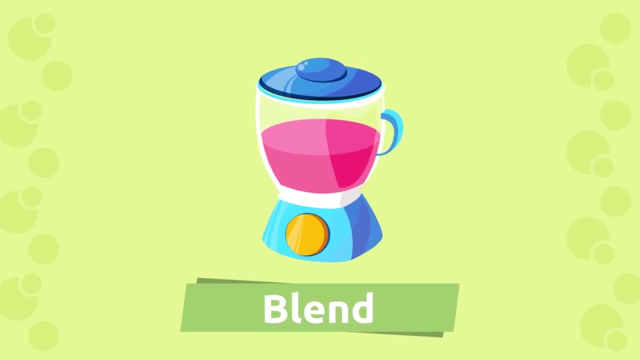 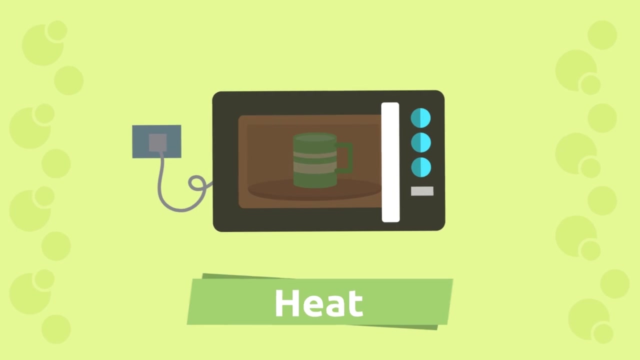 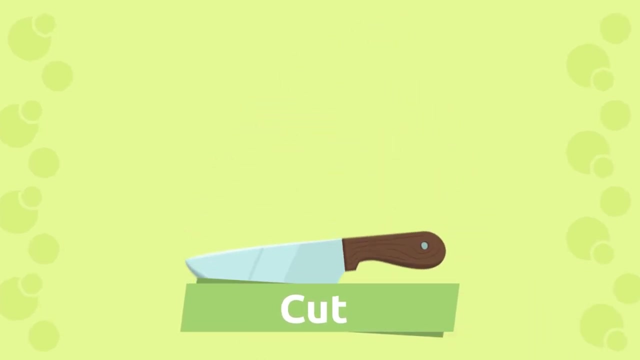 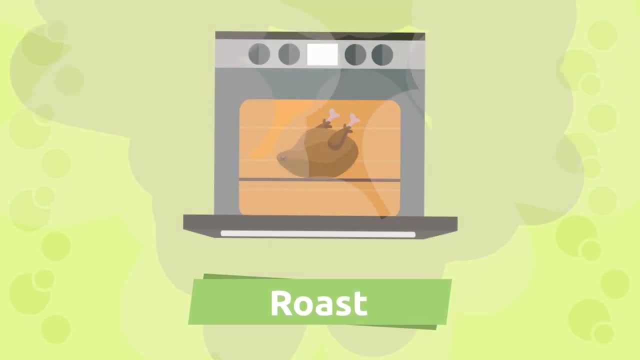 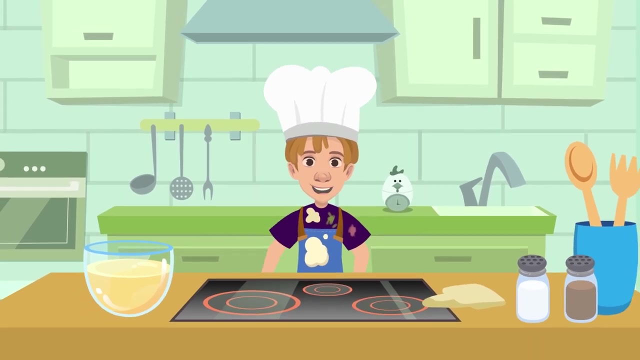 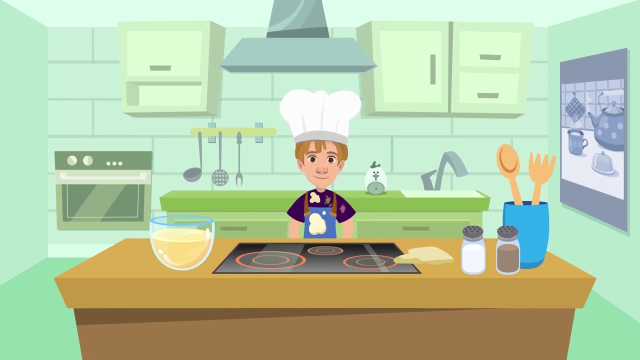 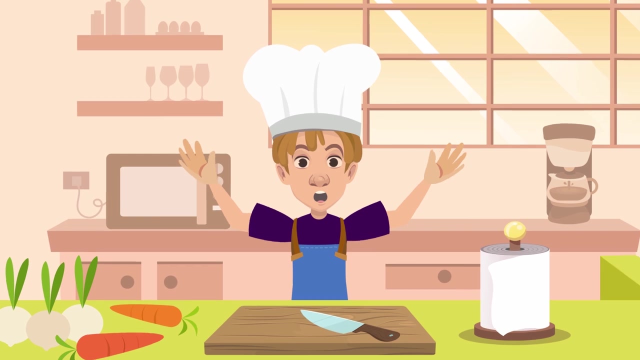 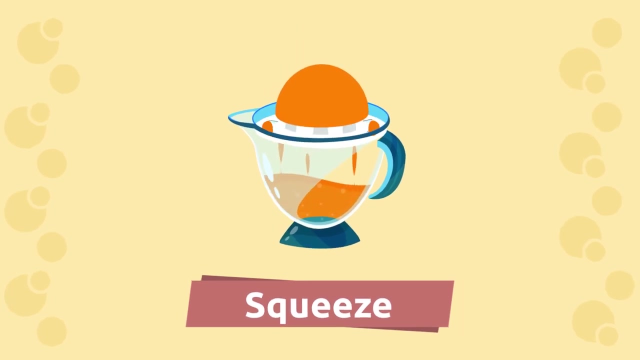 peel, chop, fry toast blend, heat, cut, weigh, boil roast. well done, friends. that's all for now. don't miss out on our next video about cooking verbs. see you soon. hi there, little chefs, great to see you again. are you all ready to learn more cooking verbs? squeeze, squeeze, repeat after me. squeeze, way to go. 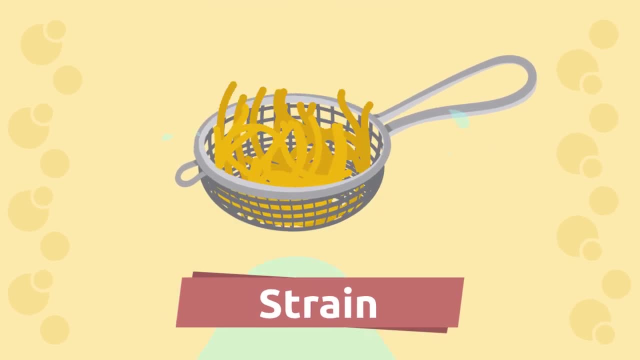 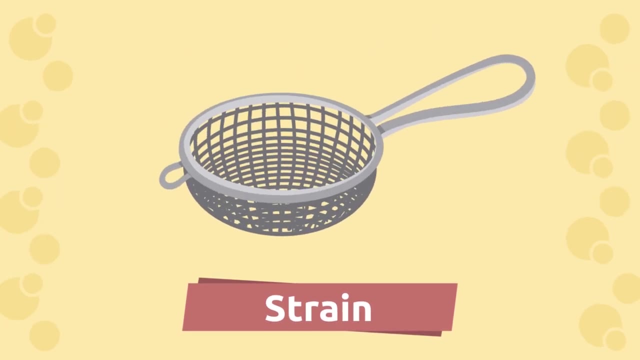 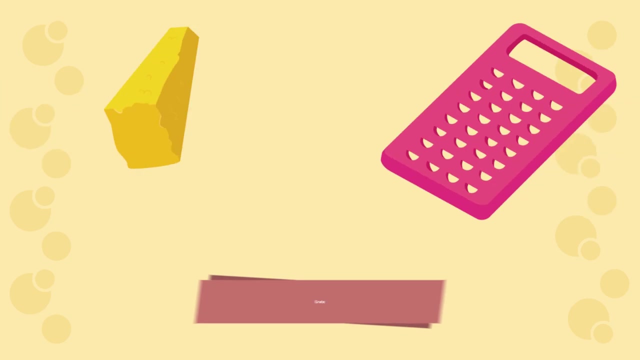 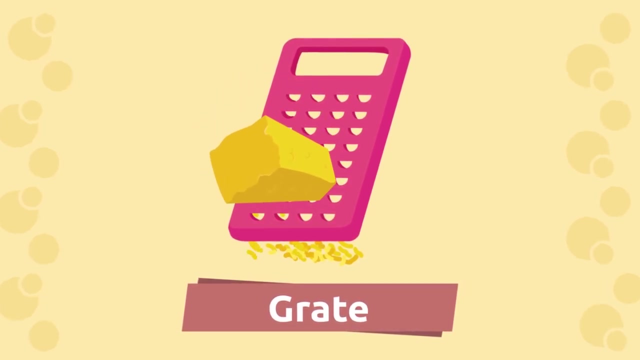 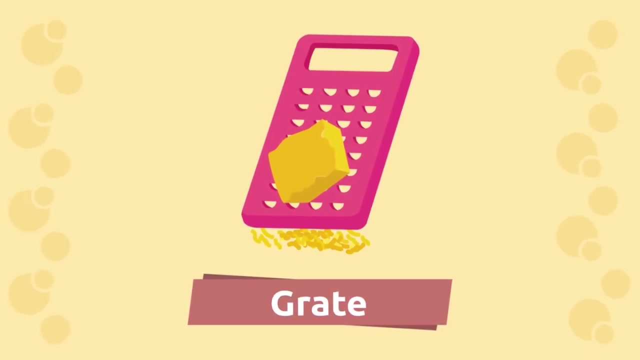 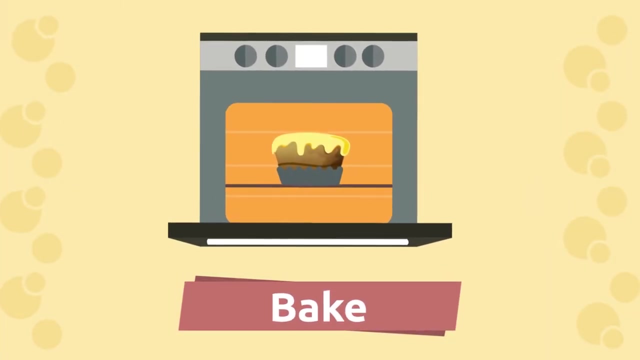 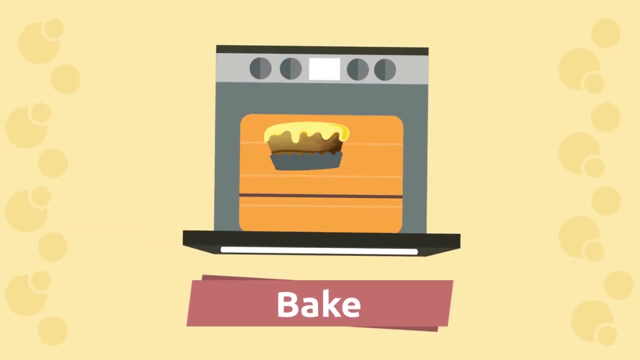 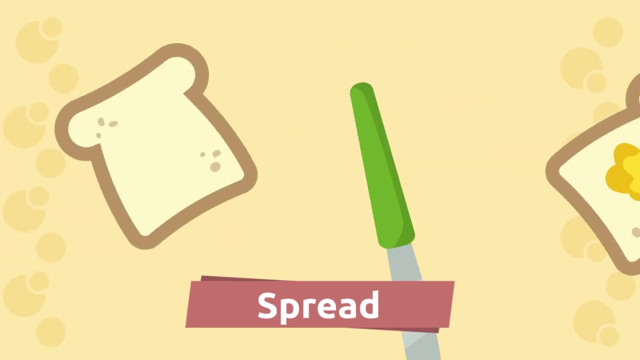 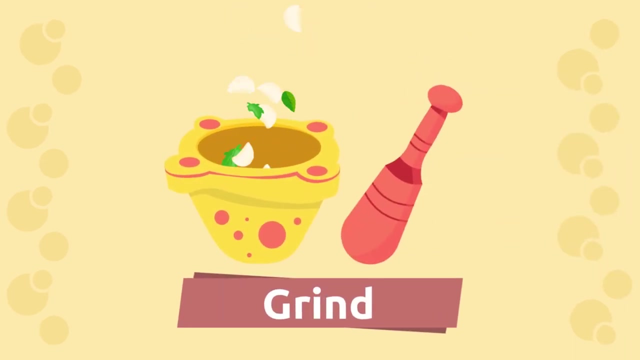 strain, strain, repeat after me: strain. awesome, great, great repeat after me, great, repeat after me, great, repeat after me. repeat after me. repeat after me: great fantastic. bake, bake, repeat after me, bake. that's it. spread, spread, repeat after me right on. grind, grind, repeat after me: grind- terrific. 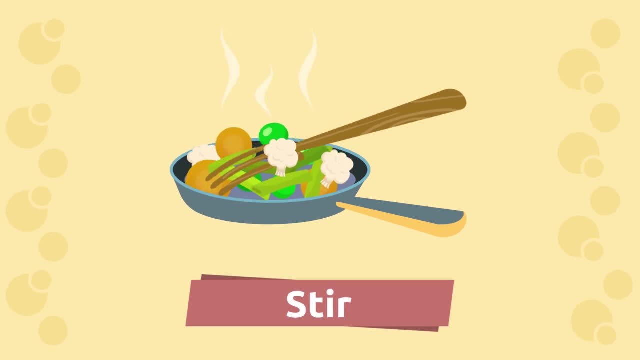 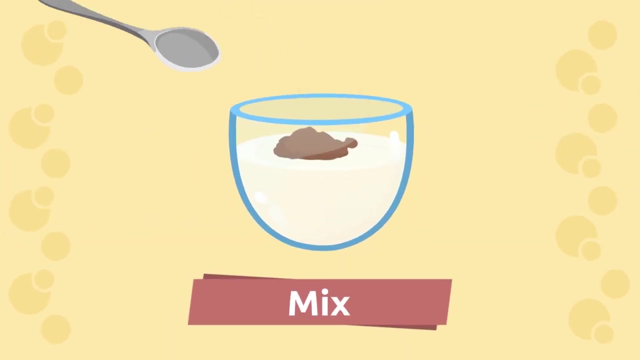 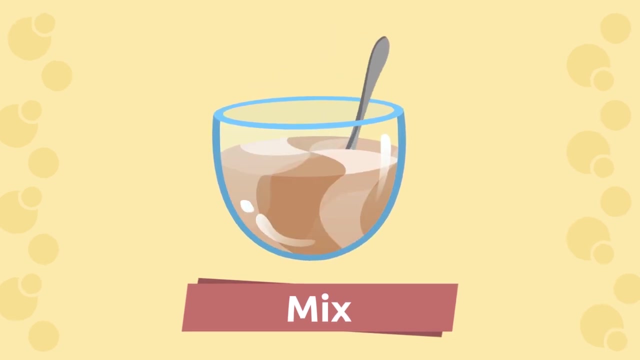 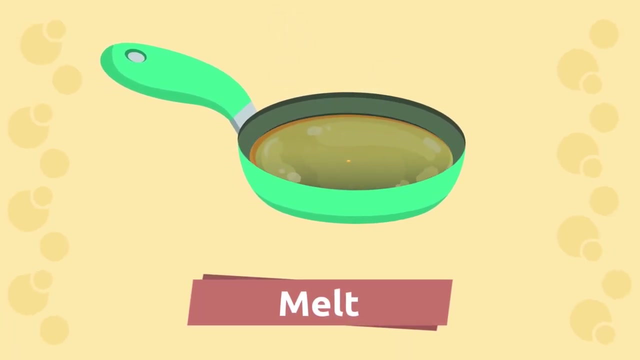 stir, stir, repeat after me, repeat after me, stir. excellent, excellent mix. mix, mix, repeat after me, repeat after me. mix. good job, good job. melt, melt, melt, repeat after me, repeat after me, melt. well done, well done pour, pour, pour, pour, pour, repeat after me, repeat after me, pour.